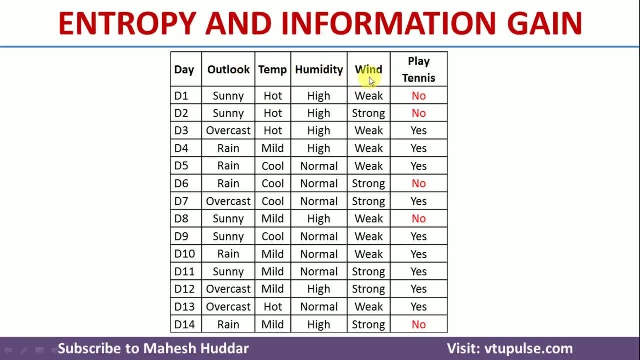 The very first thing we need to understand is how many attributes are there and what is the target class, whether it is a binary or multivalued classification. In this data, we have four attributes, like outlook, temperature, humidity and wind. Now, from these four attribute, 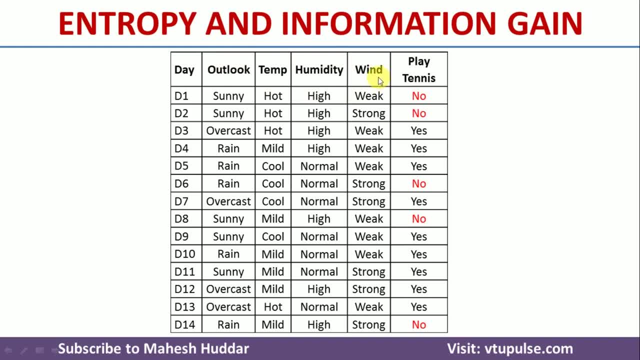 which is the first attribute I should select as the root node. Once I select a particular attribute as a root node, which is the next attribute I should select as the next level node, and so on. That is the first question we need to answer, So 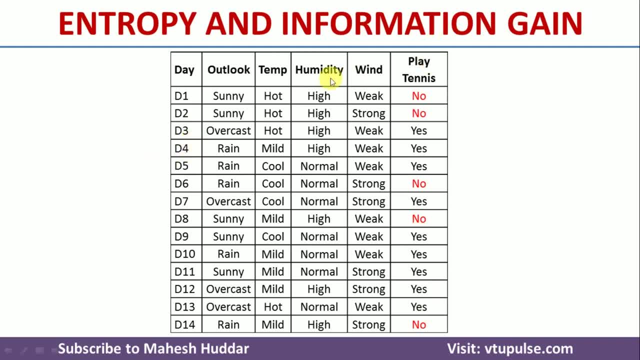 to answer that particular question, we need to calculate the information gain of every attribute. For example, what is the information gain of outlook? What is the information gain of temperature? What is the information gain of humidity and wind? Once you calculate the information gain of every attribute? 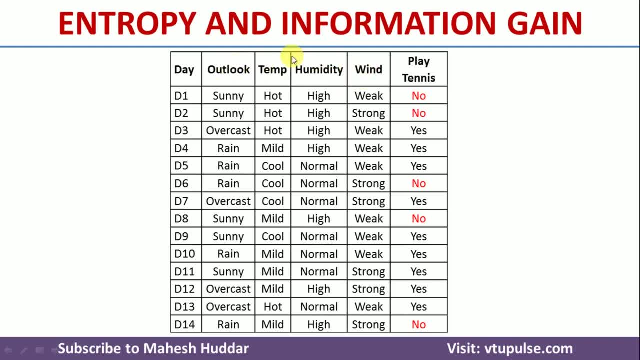 You can decide which is the attribute having maximum importance, depending on the information gain, and we can select that particular attribute as a root node at a given point of time. Now, if you want to calculate the information gain, the very first thing we need to calculate- 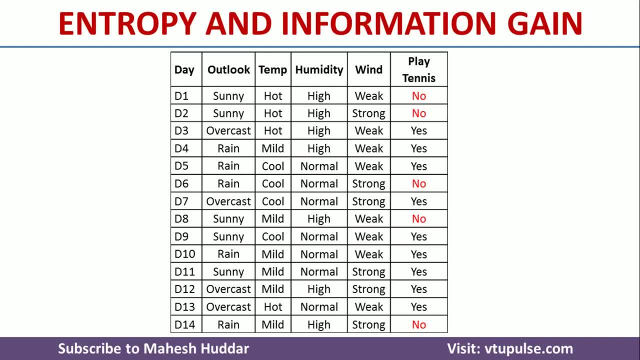 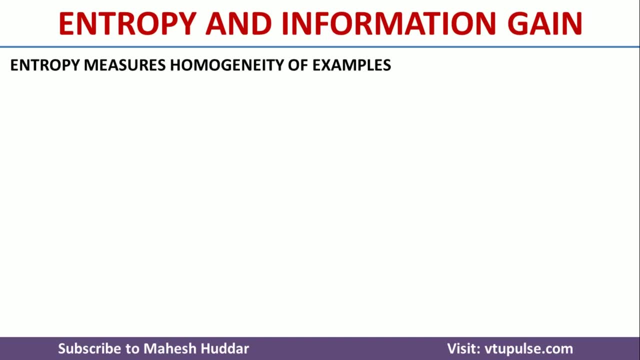 is entropy. So, given the entropy, we can calculate the information gain. Given the information gain, we can select a particular attribute as a root node at a particular instance. Now, what is entropy? Entropy measures the homogeneity of examples. That is entropy. 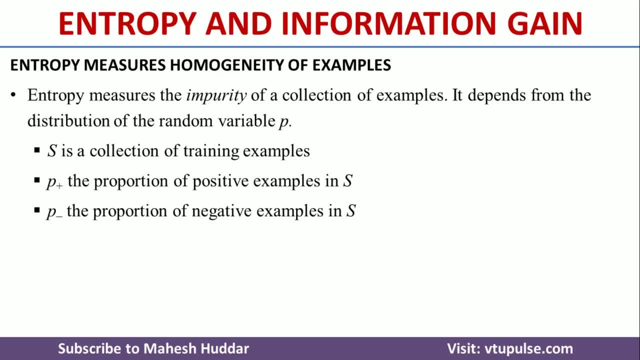 measures the impurity of collection of examples. It depends from the distribution of random variable p. For example, let us say that S is the collection of training examples. In that particular set of training examples, p plus is the proportion of positive examples and p minus is the proportion of negative examples. Let us call it p plus. P plus is: 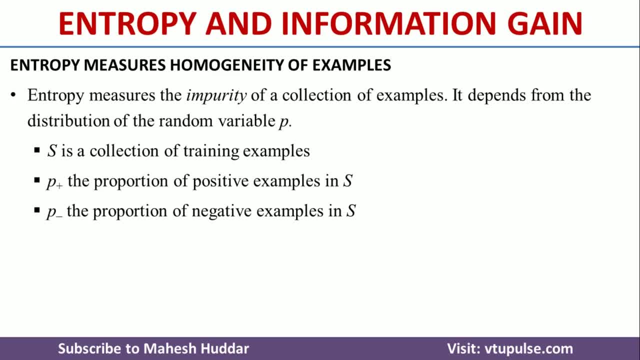 the proportion of positive examples. p minus is the proportion of negative examples. Let examples. So, given these particular data, we can easily calculate the entropy. using this particular formulae, Entropy of S, that is, the entropy of given set of examples, is always. 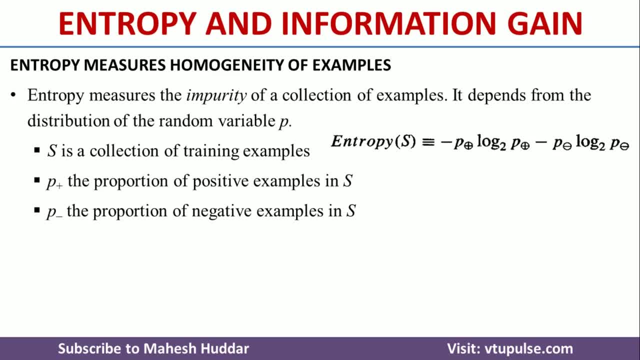 equivalent to: minus proportion of positive examples, log proportion of positive examples to the base 2, minus proportion of negative examples, log proportion of negative examples to the base 2.. So if you know this particular formulae, we can calculate the entropy of the given data set. We can use this entropy while calculating 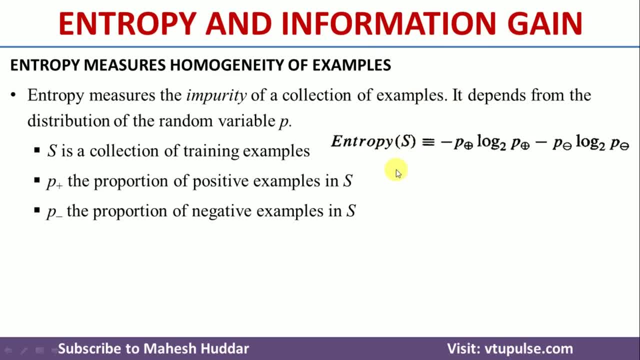 the information gain. Now we will see some of the important characteristics of entropy. For example, in this calculation I have written the entropy of 14 examples. All 14 examples are positive and there are zero negative examples. So if we get such kind of things, for example, 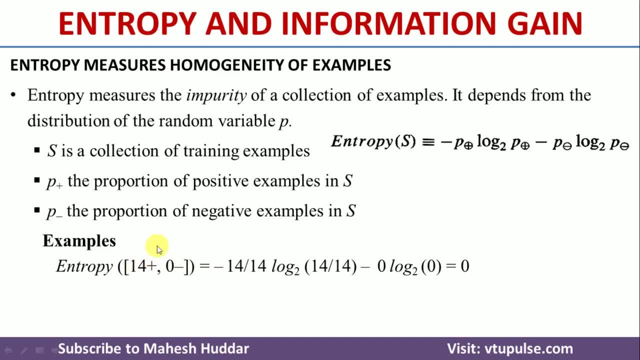 if you have only positive examples, sometimes you may get only negative examples. that is, zero positive examples and 14 negative examples. In both the cases there is no need to apply this particular formulae Directly. we can write the entropy as zero Once again if you have only positive examples or only. 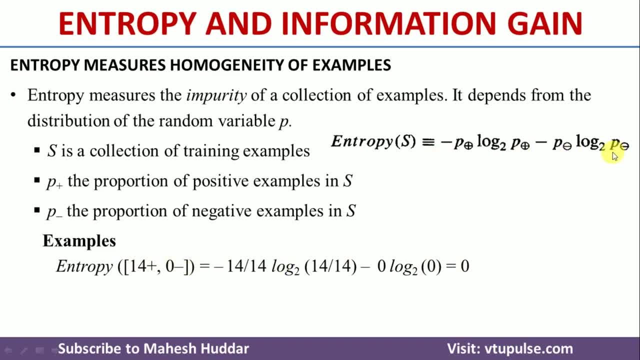 negative examples, there is no need to use this formulae to get the entropy Directly. we can write the entropy as zero here. Similarly, if you have entropy where the entropy is negative, where a combination of positive and negative examples are there, like 9 positive, 5 negative- 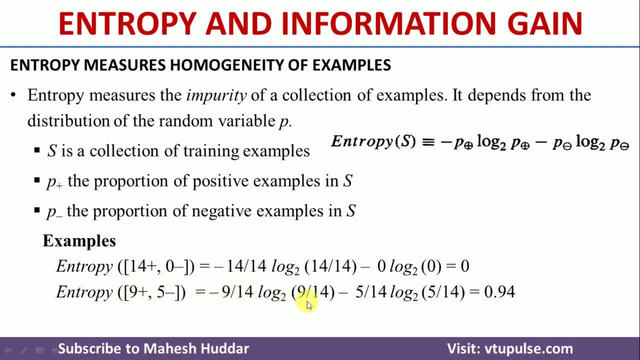 8 positive, 6 negative and so on. we need to use this formula and we need to calculate the entropy. and the third case is we have equal number of positive and negative examples, for example, 7 positive, 7 negative, 8 positive, 8 negative, 3 positive, 3 negative. that is equal. 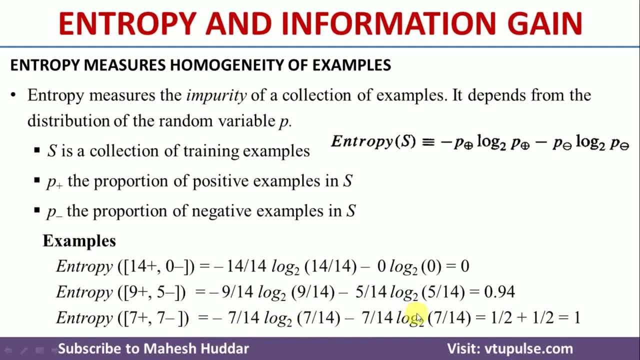 number of positive and negative examples, there is no need to calculate once again the entropy using this formula directly we can write the entropy as 1.0. so if only positive or only negative examples are there, the entropy is 0 if you have equal number of positive and negative. 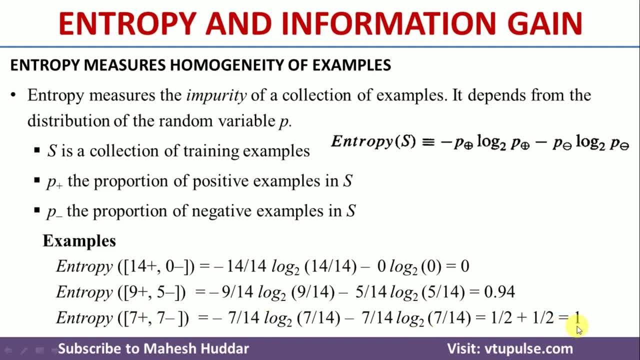 examples are there, the entropy is equivalent to 1. there is no need to calculate these two values. in the third case, if we have a combination of positive and negative examples, we need to use this particular entropy formula and we need to calculate the entropy here. so this is how i have calculated the entropy. 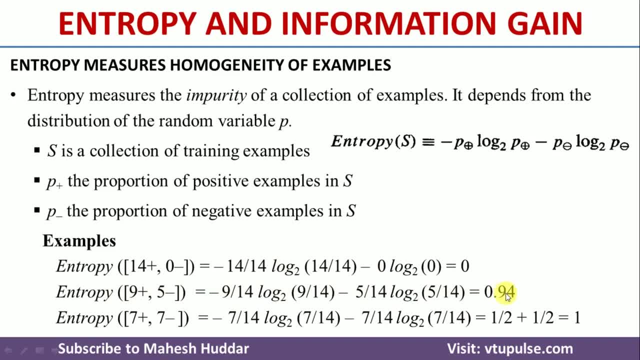 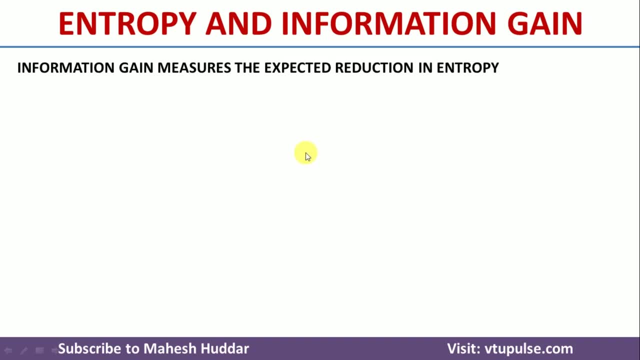 so entropy of 9 positive and 5 negative examples is 0.94 in this case. i hope you understood how to calculate the entropy of the given data. now we will try to understand how to calculate the information gain of the given data. the information gain measures, the expected reduction in entropy. the entropy measures, the impurity in the given. 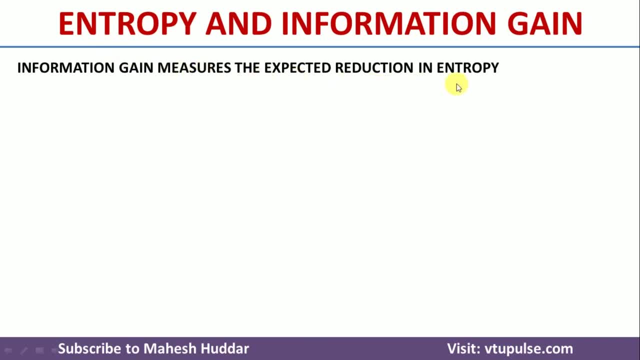 data and information gain measures the expected reduction in the entropy, that is, expected reduction in the impurity. so, given the entropy as a measure of impurity in a collection of training examples, the information gain is simply the expected reduction in the entropy caused by partitioning the examples according to an attribute. 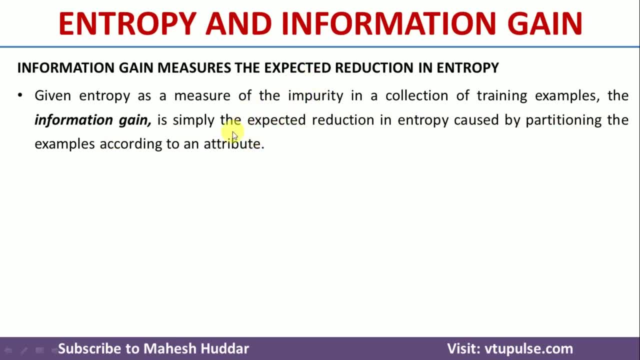 so here we have an entropy, that is, the measure of impurity. while calculating the information gain, we are trying to reduce that particular impurity. So the one attribute which has the minimum impurity, that will be considered as the important node here. More precisely, more information, the information gain, that is gain s comma a, where s is the 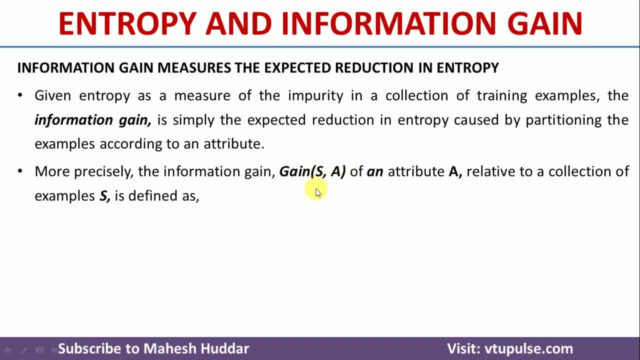 given data and a is the attribute is defined as the gain s comma. a is always equivalent to entropy of whole data set minus summation of v belongs to values of a, that is, the values of attribute under consideration. cardinality of sv divided by cardinality of s, that is: 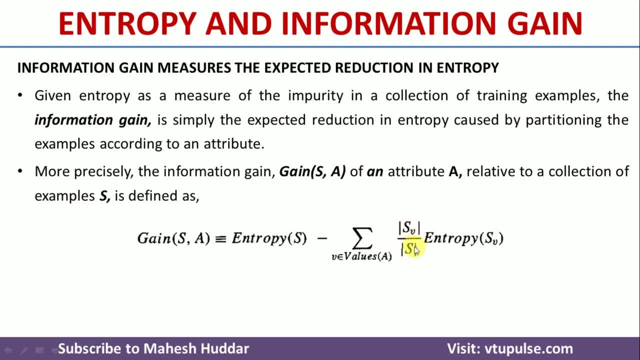 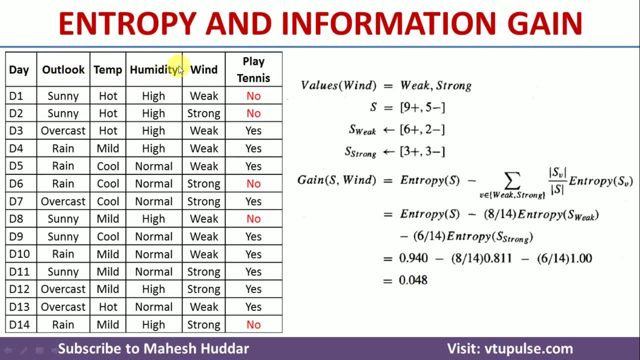 the number of times that particular value appears over the entire data set, multiplied by entropy of that particular attribute value. For example, we will take this data set. Let us say that in this particular data set We want to calculate the information gain of wind. There are four attributes we need. 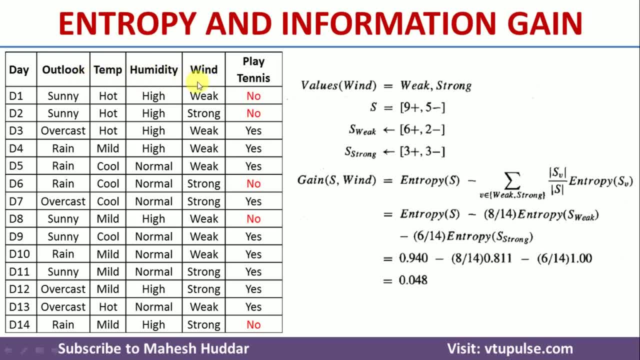 to calculate the information gain of all four attributes while drawing the decision tree. In this case, I will be showing how to calculate the information gain of wind here. The very first thing what I need to do is I need to write what are the possible values for wind. 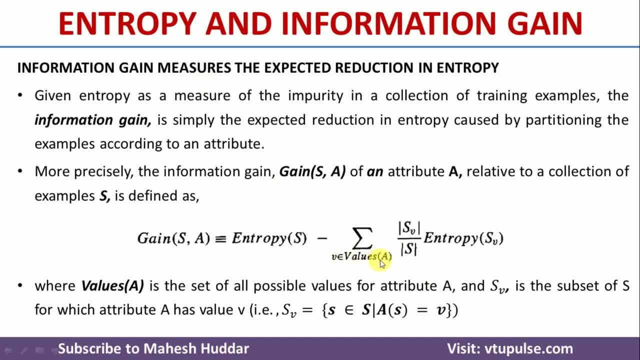 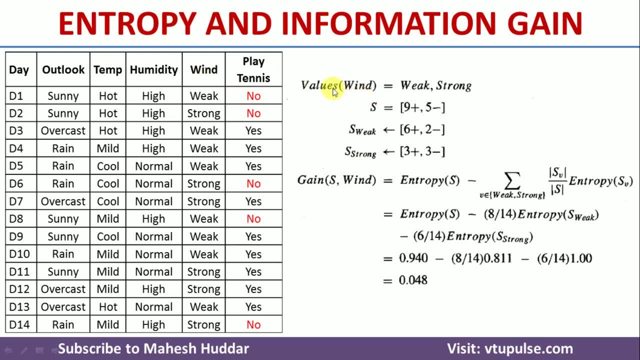 because I will be using that particular thing here. V belongs to values of a, that is, a is the attribute. in this case the attribute is wind here. So first I will write it: how many possible values are there for wind? Values of wind are, we can see here: weak is the one possibility, strong is the another. 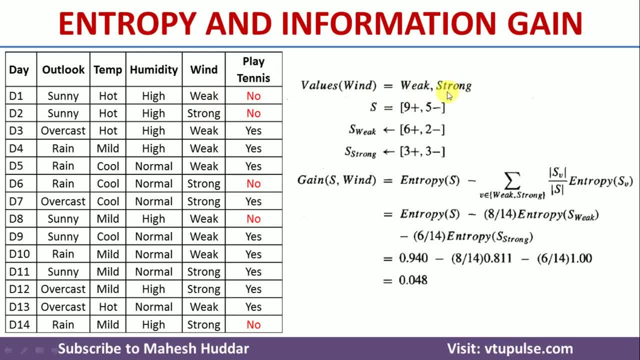 possibility. So I have written those two things here. Now, from this particular entire data set, how many positive examples are there and how many negative examples are there we need to find. You can see here, if you look at this target function, I have marked the. 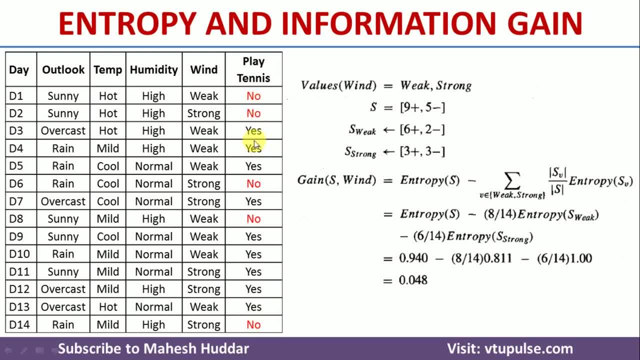 negative examples, as with a red color, and the positive examples, as black color. So if you count these things, 1, 2,, 3,, 4,, 5,, 6,, 7,, 8,, 9,, 10,, 11,, 12,, 13,, 14,, 15,, 16,, 17,, 18,- 19,, 20,, 21,, 22,, 23,, 24,, 25,, 26,, 27,, 28,, 29,, 30,, 31,, 32,, 33,, 34,, 35,, 36,, 37,, 38,, 38,, 38,, 39,, 40,, 40,. 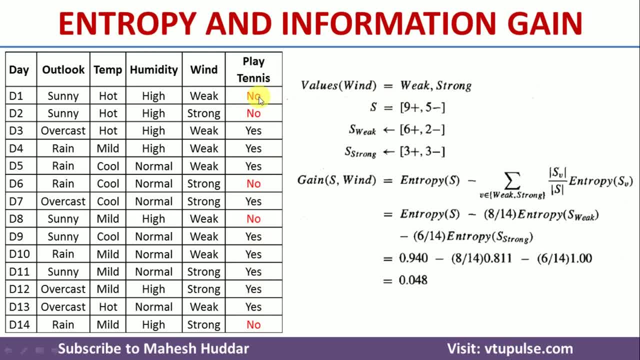 31,, 42,, 34,, 35,, 36,, 37,, 38,, 39.. So 9 positive examples are there. If we count the negative examples- 1,, 2,, 3,, 4, and 5, so 5 negative examples we have. So this is the first thing. 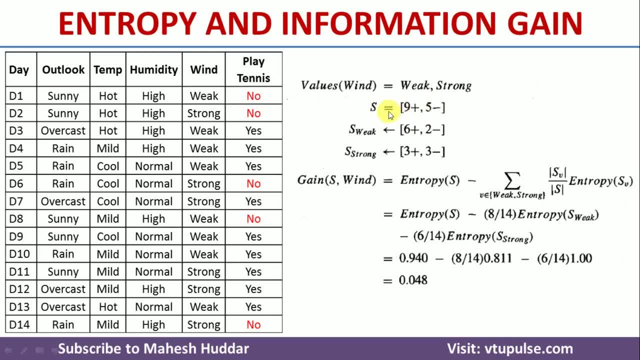 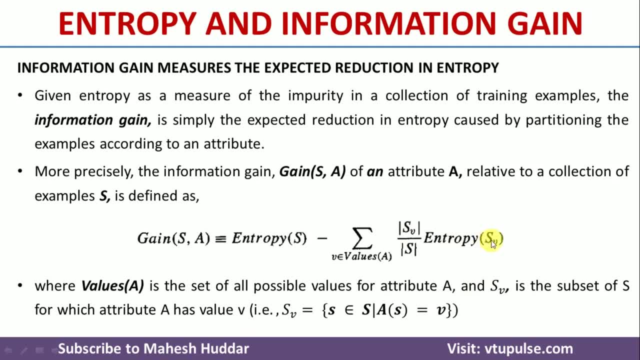 we need to write This is with respect to the entire data set. The second thing is the entropy of individual attribute values. we need to find that is written here: Entropy of SV, that is, a entropy of first value, entropy of second value, and so on. So in this case, 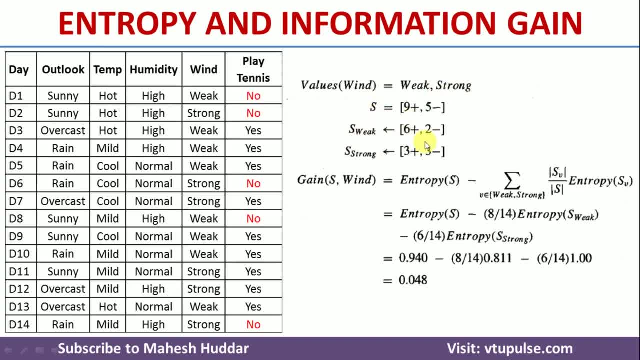 there are two values are there, that is, weak and strong. So we need to calculate the entropy of weak and strong. so first of all, we need to count how many positive examples are there and negative examples with respect to weak, and how many positive and negative examples with respect. 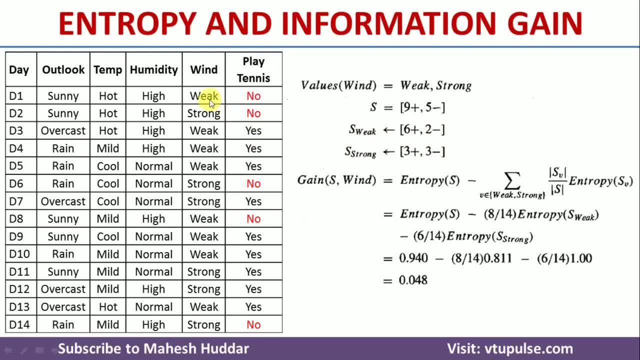 to strong here. now, if you consider only weak, that is yes, weak there are. we need to first count how many weak are there. so first one is this: second, third, fourth, fifth, sixth, seventh and eight. there are eight possible examples where weak is present. out of these particular eight examples, how many? 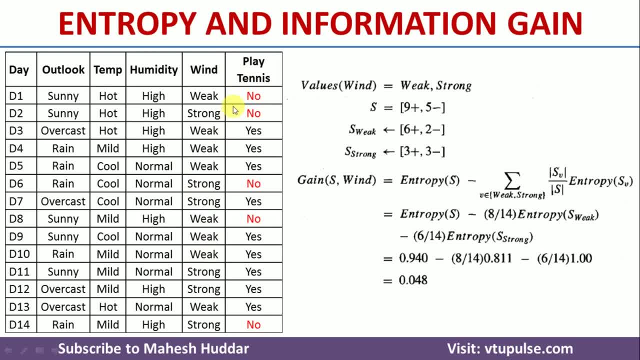 positive examples are there? how many negative we need to find? if you find it weak, here is negative, second one is positive, third is positive, fourth is positive and fifth is negative, sixth is positive, seventh is positive and eighth is positive. so totally six positive are there and two negative. 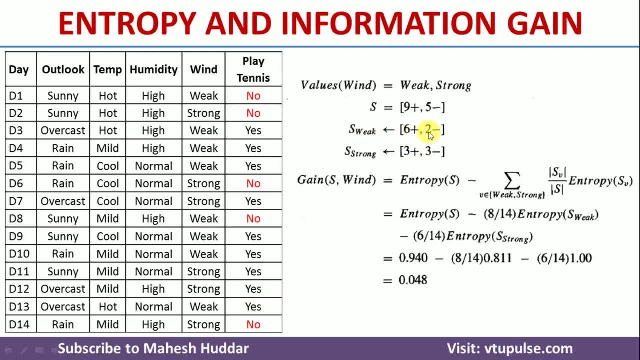 values we have. so, yes, weak is equivalent to six positive and two negative. yes, strong is equivalent to three positive and three negative. we just count it out. yes, strong is negative here, strong is negative here, strong is positive, strong is positive, strong is positive and strong is negative. so three negative and three positive we have here. so, given this particular data, we can 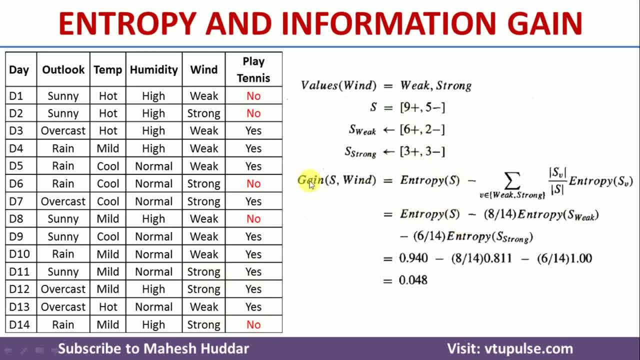 put this: we can calculate the entropy and then we can find the gain. so gain of s given for this wind is equivalent to entropy of s minus. summation of phi belongs to weak and strong, that is, the values are weak and strong. cardinality of sv divided by cardinality of s entropy of sv. so 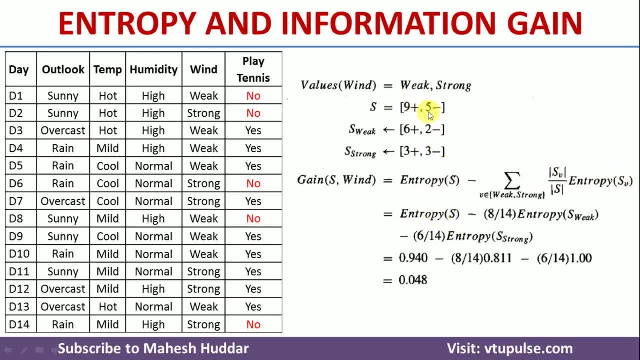 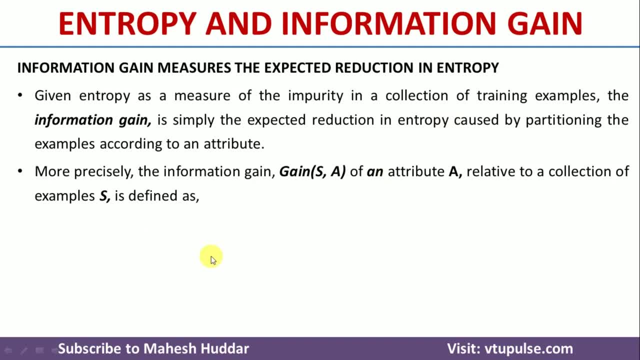 entropy of s we need to find, that is, we have this particular number of positive and negative examples here. so, if you find it out, in the previous slide i have shown 9 and 5. if you have those values, what is the entropy? the entropy we have calculated it is already equivalent to 0.94. 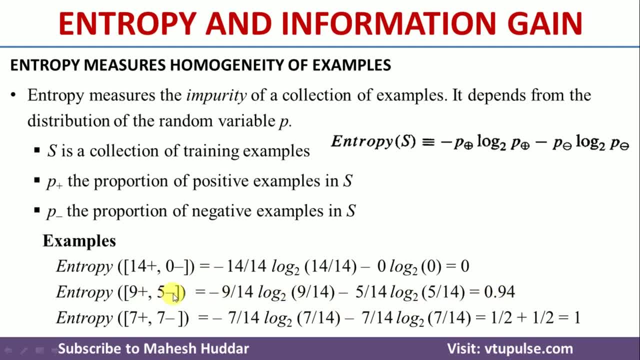 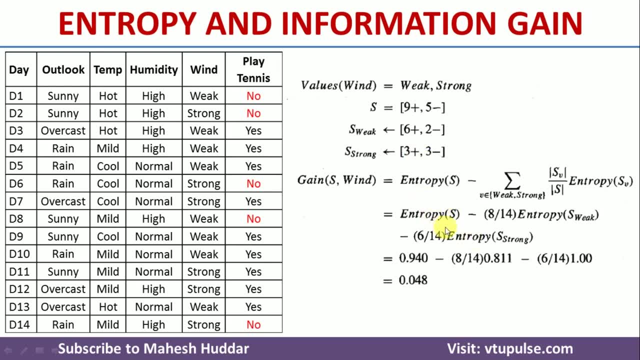 so i have not calculated it again. so if you have 9 positive and 5 negative examples, the entropy is 0.94, so that one i have calculated in the previous slide. you just check it out. so that is 0.94. now summation term. we need to write here: this particular summation term is sv. 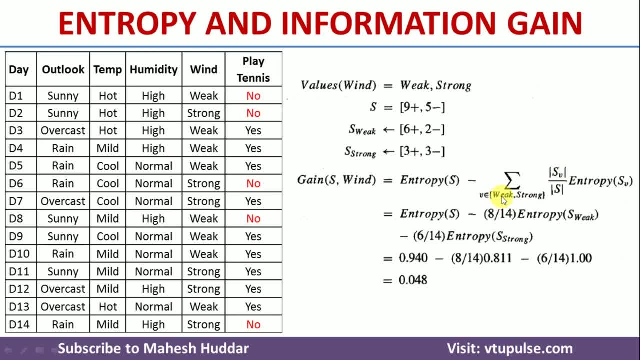 that is how many number of times weak is appearing if you just check it out: 6 plus 2, 8 times it is appearing out of cardinality of s, that is, cardinality of s is 9 plus 5, that is 14, 8. 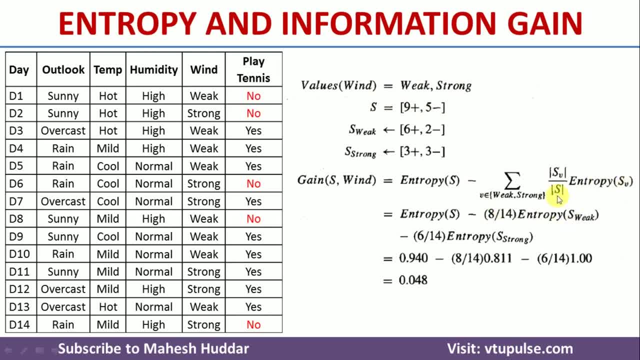 divided by 14. entropy of sv, that is s weak minus. again, how many number of times strong is appearing? 3 plus 3, that is 6, 6 times it is appearing out of 14 examples. entropy of s: strong, as i said earlier. entropy of s, that is 9 plus and 5. 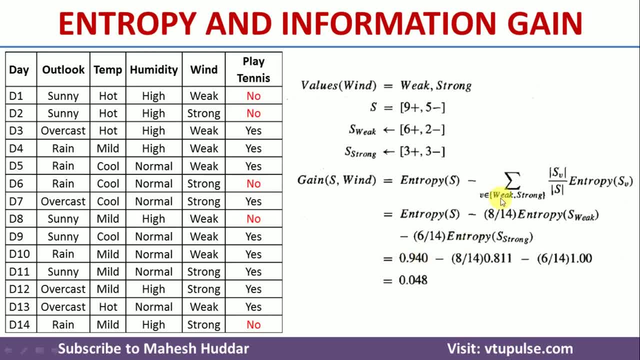 negative. we have already calculated 0.94 minus 8 by 14. as it is, we need to calculate the entropy of sv with the 6 and 2, which is equivalent to 0.811 minus 6 by 14. entropy of strong, that is. 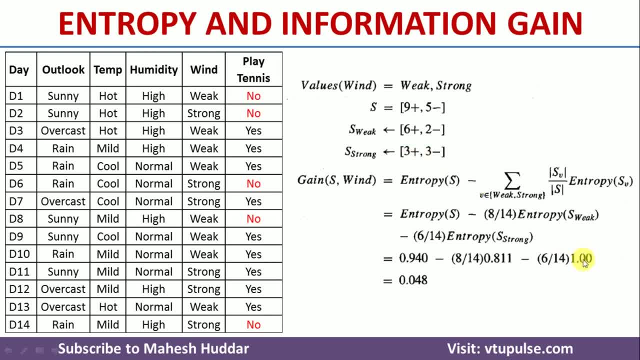 3 plus and 3 minus. if you have equal number of positive and negative examples, i told you it is directly equivalent to 1.00. so calculate this particular equation, you will get. the gain of wind with respect to given data is 0.048 in this case. so this is how we can calculate the.